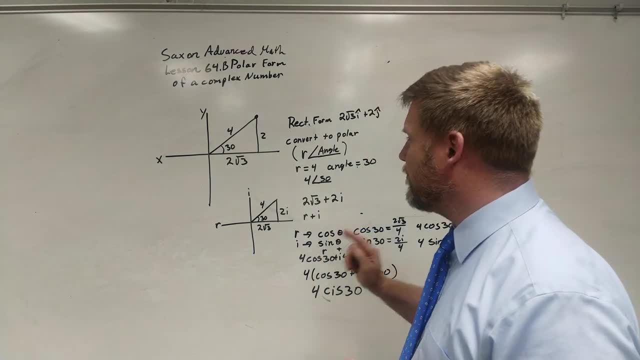 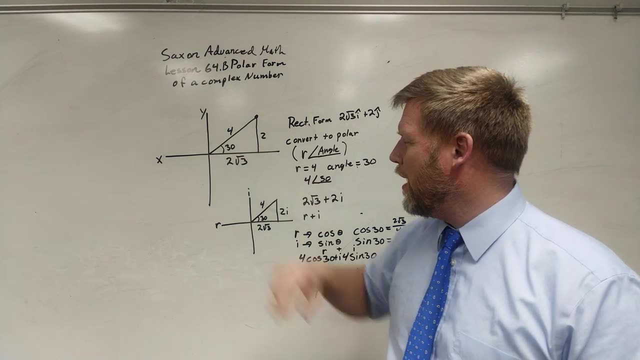 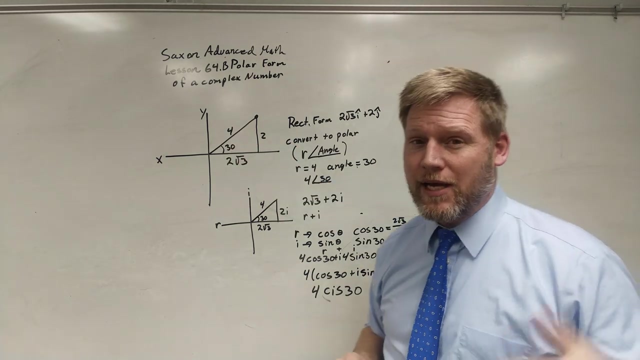 Let me explain this: why we're going to do this. If I wanted to find out what this angle was, I would say the opposite, over the hypotenuse right, which is the sine, and I would say: the sine of theta equals 2 over 4, with a sine of 0.5 is 30, and that's where that number came from. 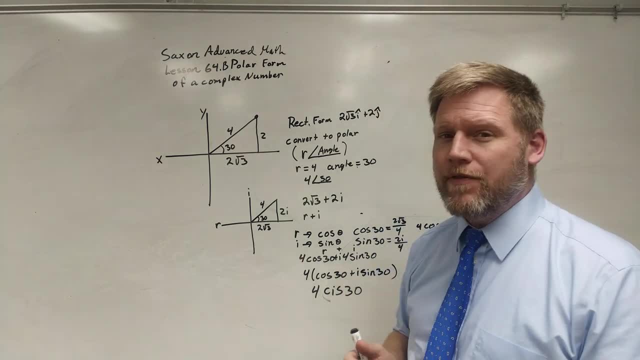 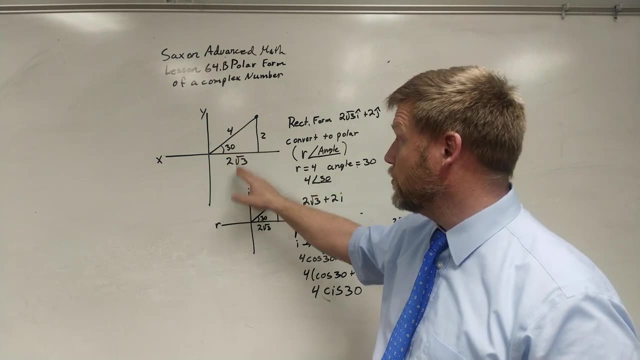 Now they're giving us this number, They're already putting it in there, But we've done this conversion where we were only given these two, and we find this angle. So we're using the sine or using the cosine, depending on our given values, to figure this out, and we can do either one. 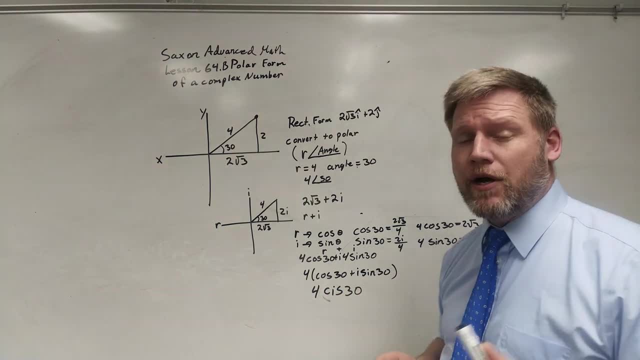 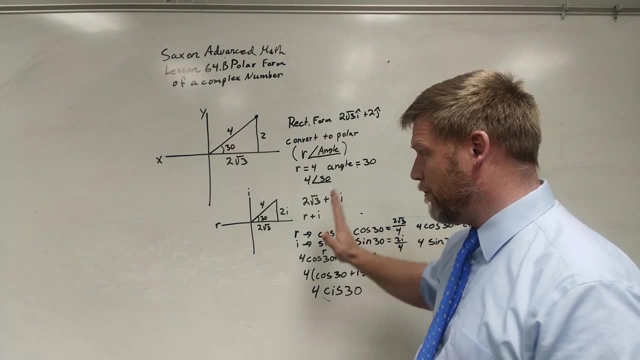 Now we're going to employ that same thought process when it comes to the complex plane or the imaginary plane. Here I have 2 root 3 plus 2i. Now keep in mind- this is from the first part of this lesson- that this is the real plus imaginary number, right? 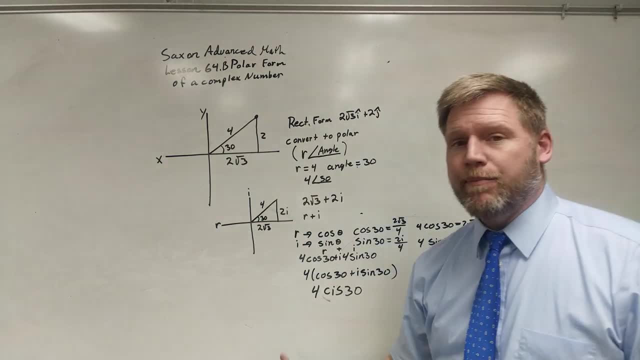 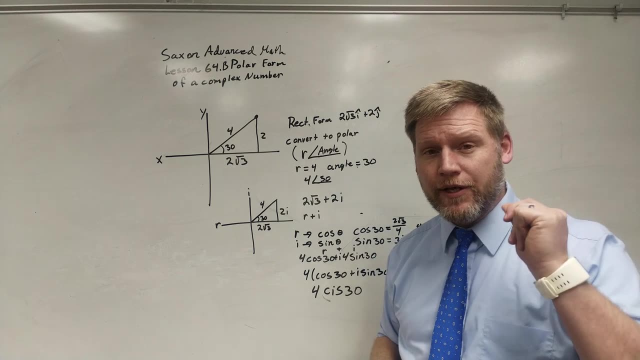 So I have the real number and the imaginary number going vertically, And the real number is 2 root 3. And the imaginary number is 2i, And we were able to get to that very quickly. There it is. It's done right Easy. 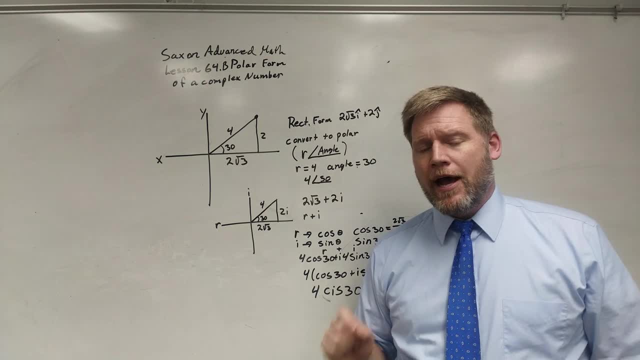 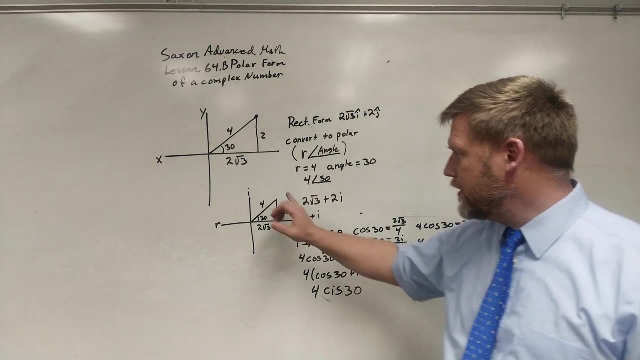 And we can define this point In rectangular format. that's what it is. However, in imaginary number in polar form, we run into an issue. This is the combination of real and imaginary numbers. right, That's what that is. 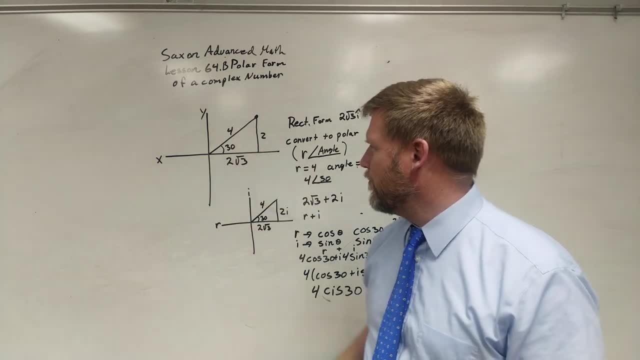 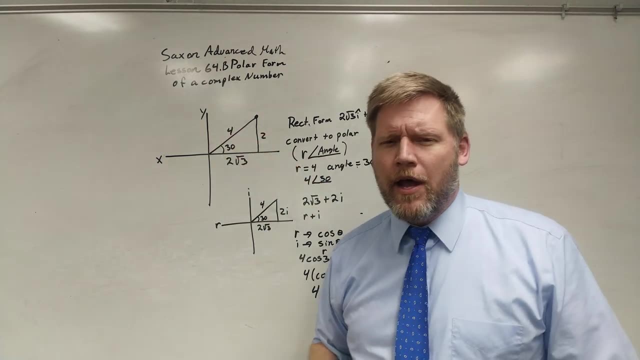 This is the combination of the x and the y, right. In fact, if we realize it's a right angle, right, We could use Pythagorean theorem and solve this And we would have gotten that number. And it works out really well. 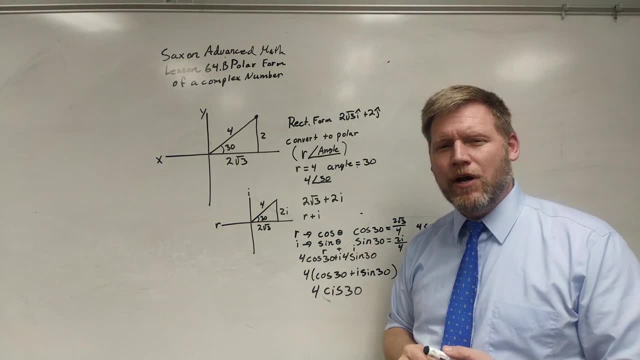 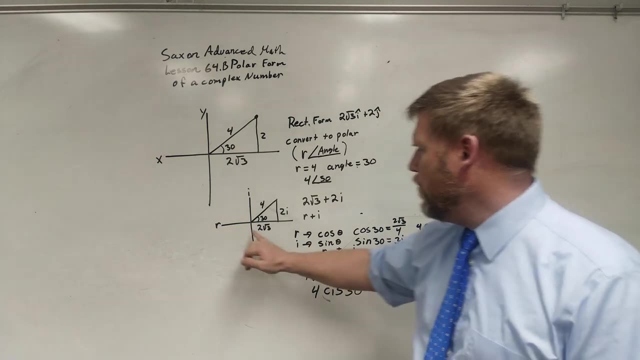 However, how do you combine a real and imaginary number when they're not like terms? You can't add them up. What are we going to do? So let's go ahead and define that. We know that this is the real direction. This is the imaginary direction. 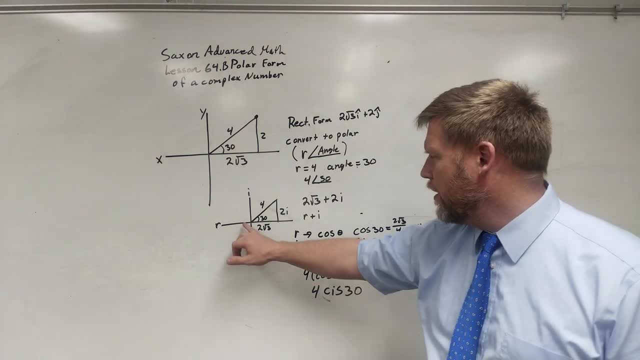 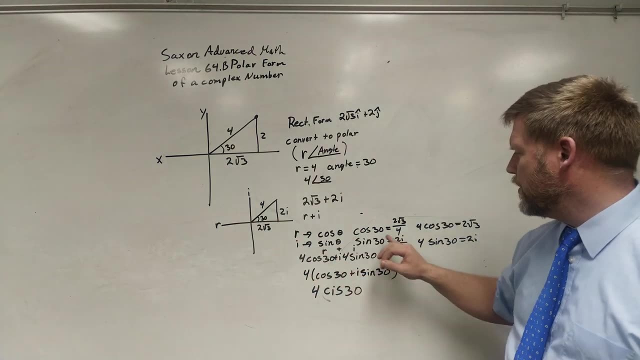 So we're going to say real is going to be dependent upon this number, would be dependent on the cosine right Adjacent over hypotenuse. Well, that's easy. What's the adjacent Cosine of 30 is, for this one, adjacent over hypotenuse? 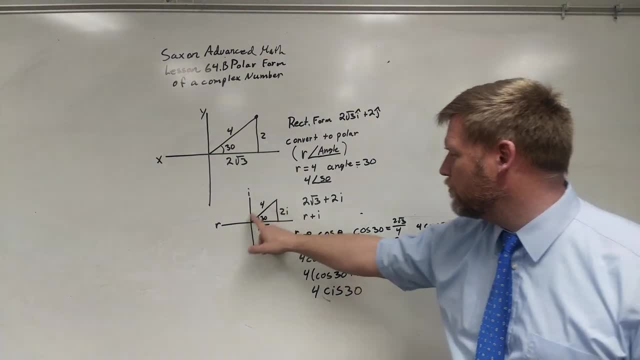 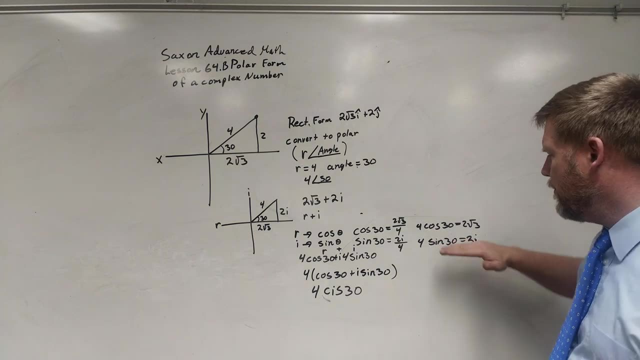 If I wanted to say, well, how could I define just the real direction of 2 root 3?? I could say, well, 2 root 3 is equal to 4 cosine theta. That all of a sudden makes a little more sense to me. 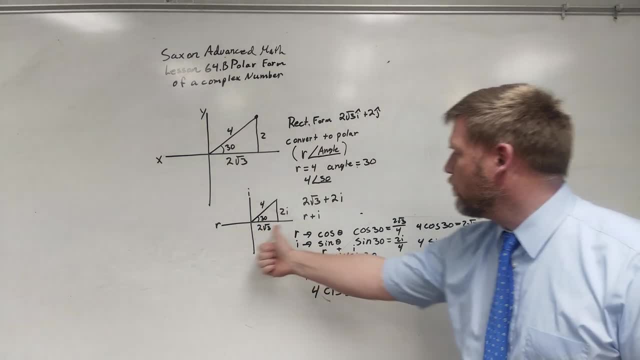 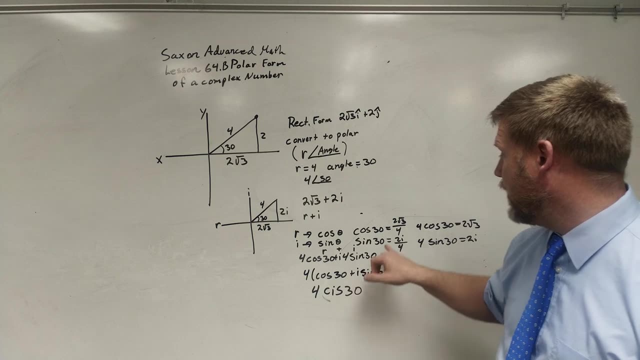 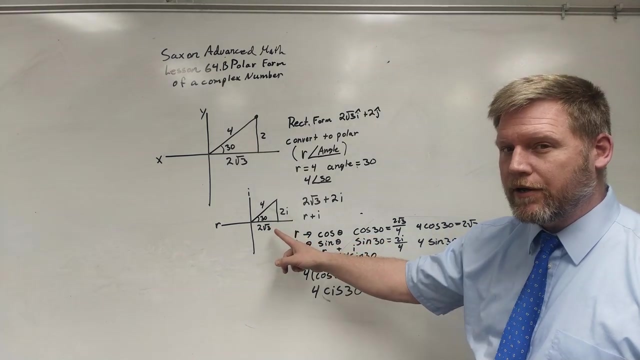 I can define that. That's how far right that is in correlation. Putting this hypotenuse in, the length is 4 cosine theta And I can define the sine of 30 that direction. That's how I would define this, using only the real number line. 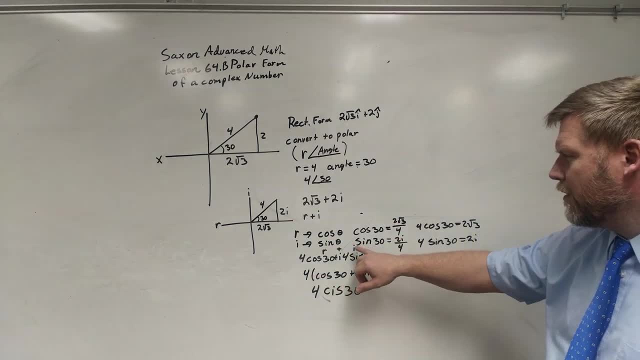 Now, when I define the sine or the i, the imaginary, I'm going to do the same thing. I'm going to use opposite over hypotenuse, which is the sine, And that's going to be 2i over 4.. 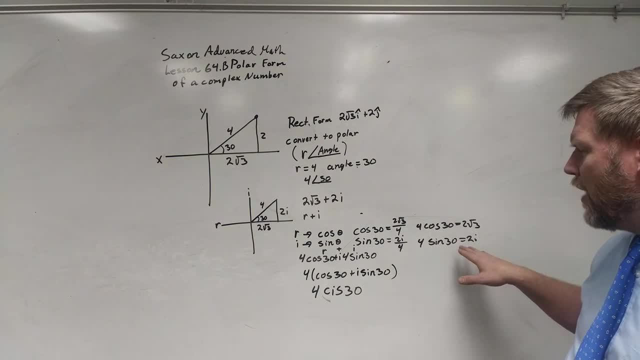 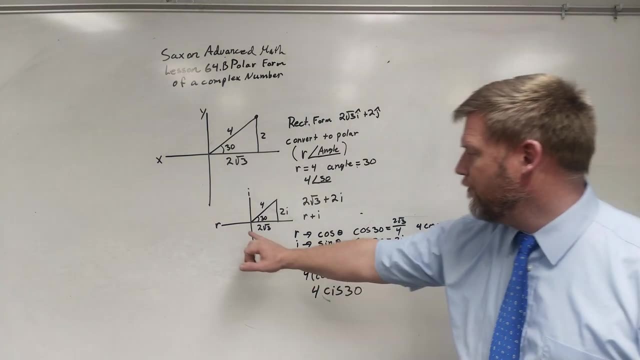 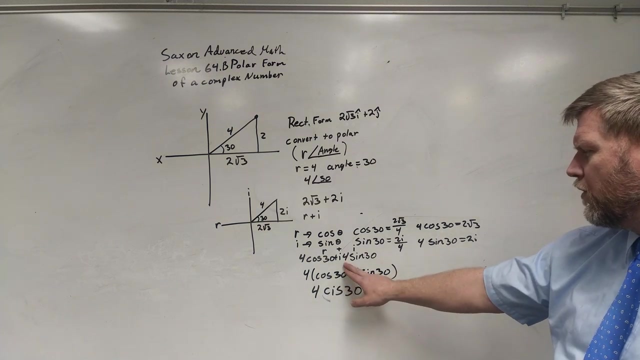 4 sine 30 is going to be equal to 2i. When I start plugging these in, I realize that I could define this right here as the addition of how far right I'm going, how far up I'm going, And therefore I could say 4 cosine of 30 plus i, 4 sine of 30. 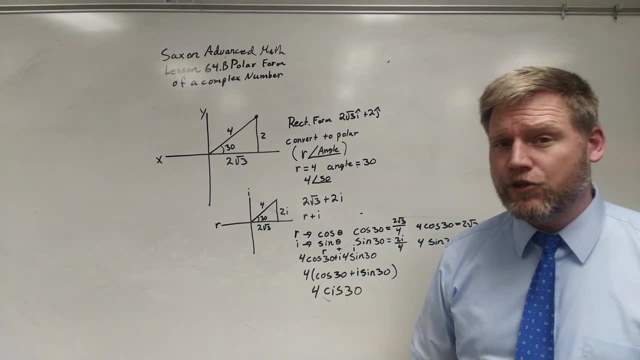 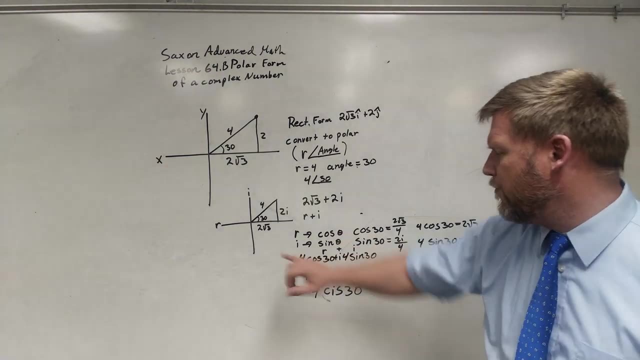 And I'm putting that i in there to tell me that it is on the imaginary direction. And when I do so I realize that this has both 4s in it. So if I factor that 4 out to the front, I'll get 4 times the cosine of 30 plus i sine of 30.. 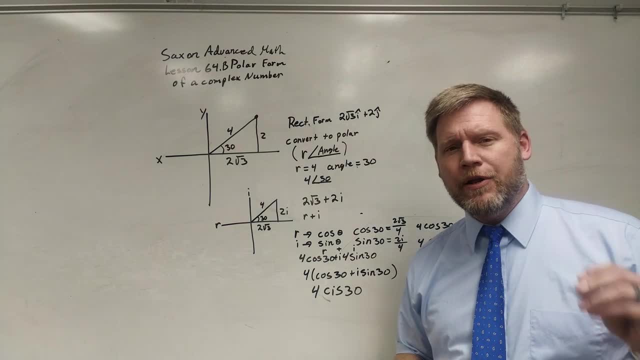 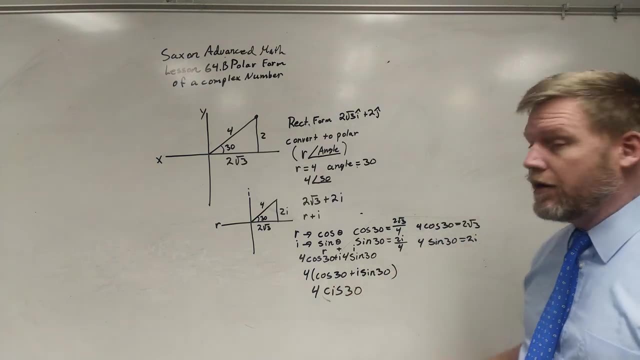 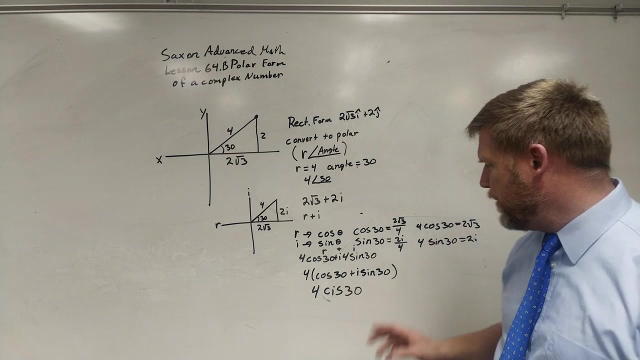 Now this right here is a 2. This is a common form of writing this in polar. Unfortunately, it gets really old writing cosine 30 plus i sine 30. Cosine of theta plus i sine theta, over and over and over. 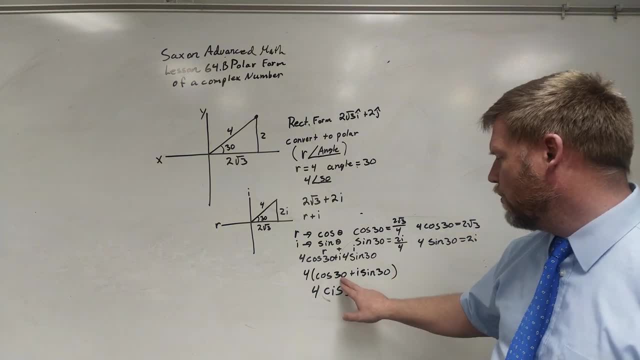 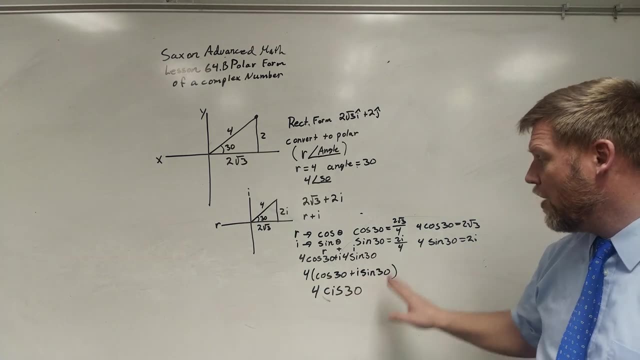 And because a couple of things. This will always be cosine, This will always be sine, This will always be the same angle as this one. It doesn't matter if I'm in second quadrant, It works out that way. third or fourth. 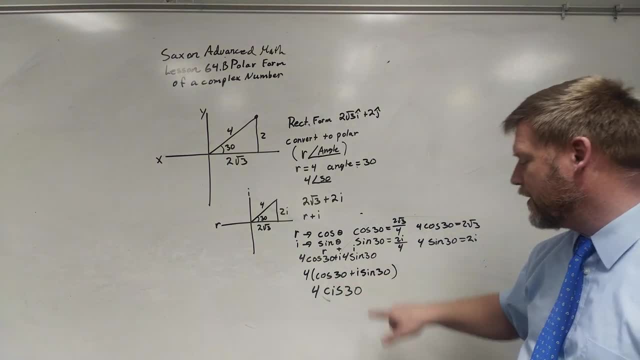 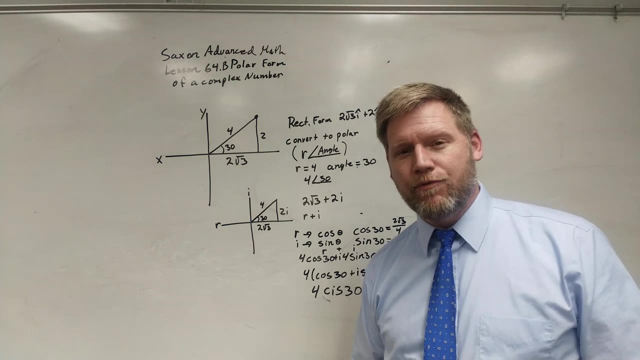 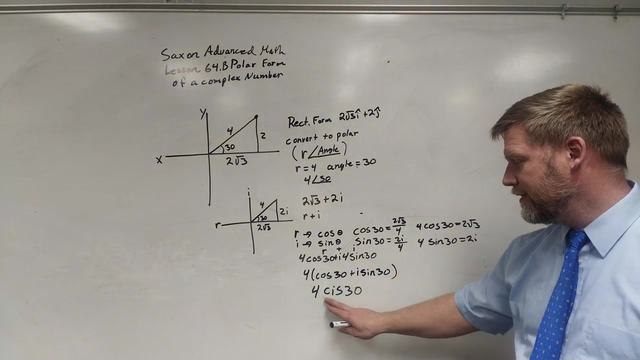 It always ends up being: these two angles are the same: Cosine plus i sine. So, like we do everything else in math, when we have something that happens a lot, we come up with an abbreviation for it. The abbreviation for cosine theta plus i sine theta is cis and the theta.